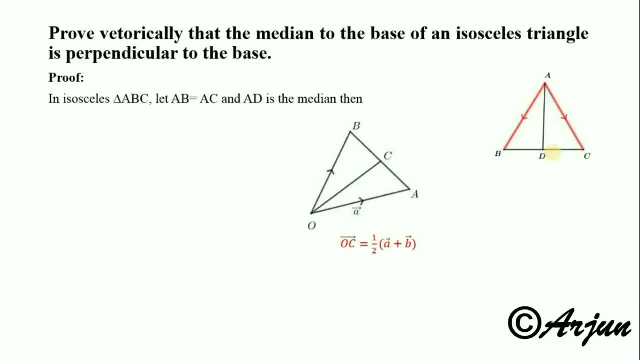 so we have to apply this midpoint theorem which we have studied earlier. so if AB is the midpoint C, then the position vector of OC is 1 by 2 A vector plus B vector. so if B is the midpoint of BC, then the position vector of AD is equal to 1 by 2 AB plus AC. 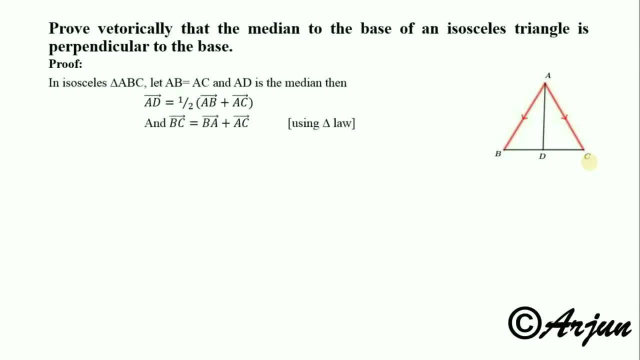 so if B is the midpoint of BC, then the position vector of AD is equal to 1 by 2 AB plus AC. so if B is the midpoint of BC, then the position vector of BC is equal to 1 by 2 A vector plus AC. 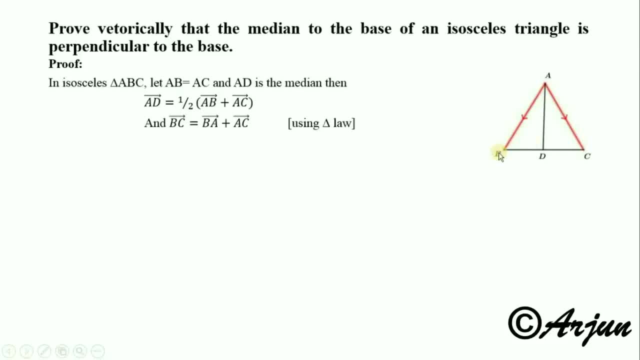 so if B is the midpoint of BC, then the position vector of AD is equal to 1 by 2 AB plus AC. now we have to apply this midpoint theorem to the vector addition. BC is equal to BA plus AC. now we have to show the dot product of DA and DV. 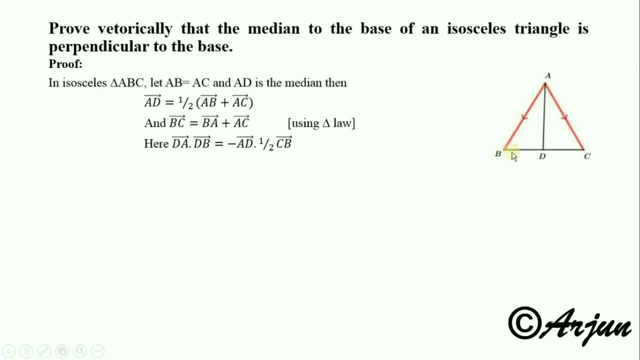 So in this point D, AD and BC are perpendicular, So we will write DA and DB dot to dot here. If we arrange DA it will be minus AD Dot. DB is 1 by 2 CB, DB is D midpoint, So we can write 1 by 2 CB in place of DB. 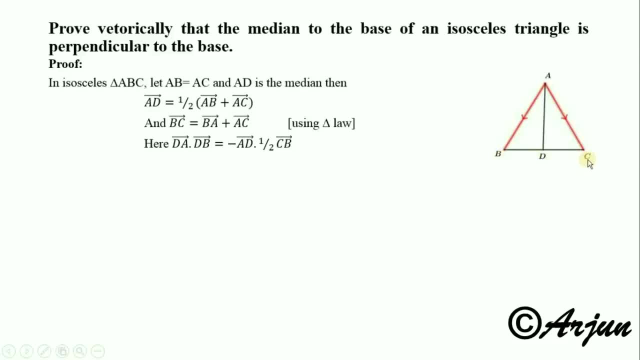 We can't write BD because direction between D and B is same, So we will write 1 by 2 CB here. If we arrange this, it will be 1 by minus AD as it is, And 1 by 2 as it is. If we arrange CB, it will be BC. 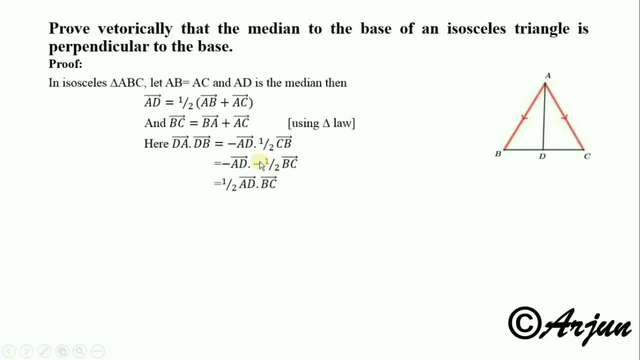 It will be negative vector, it will be minus. before, If we arrange, it will be 1 by 2, AD, dot, BC. Now let's see: Keep the value from above, 1 by 2 multiplied by 1 by 4, In place of AD, AB plus AC. 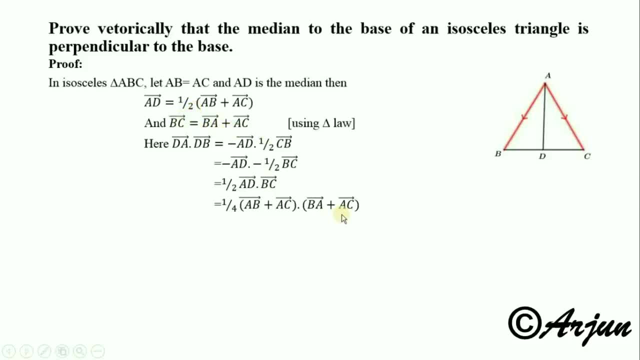 In place of BC. BC is equal to BA plus AC, So we will keep the value of AD and BC 1 by 4 as it is: AB plus AC as it is. If we take AC as it is And if we arrange B as it is, it will be negative vector. 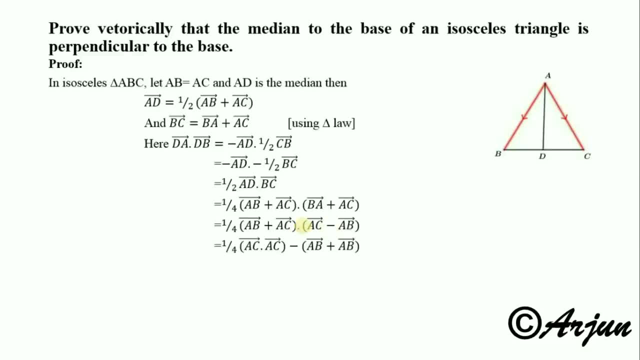 So it will be minus AB. It is in the form of A plus B, A minus B, So it will be AC square minus AB square. AC square will be AC dot AC. So we will write AB dot AB. So we will write 1 by 2: AC vector square minus AB vector square. 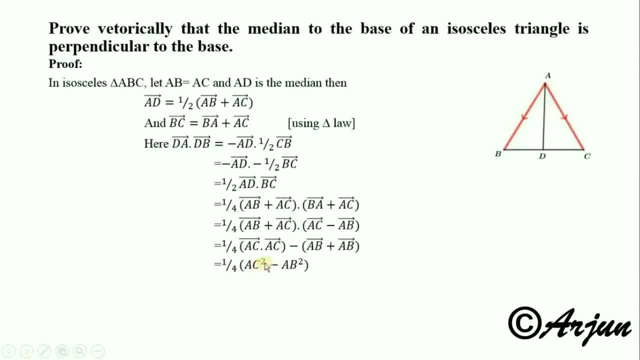 This AC vector: square and AC square is same. We have discussed this earlier Vector A square and A square is same. It is in the form of magnitude. So we will write AC square and AB square 1 by 4 into AC square minus AB square is equal to 0. 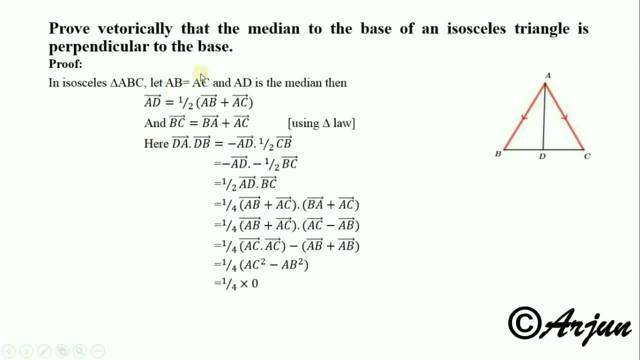 Here we have laid: AB is equal to AC, AB is equal to AC, Isoceous angle is equal to side, So this is equal. AC and AB is same, So AC minus AB is equal to 0, AB is equal to 0. Now, what it provides is: 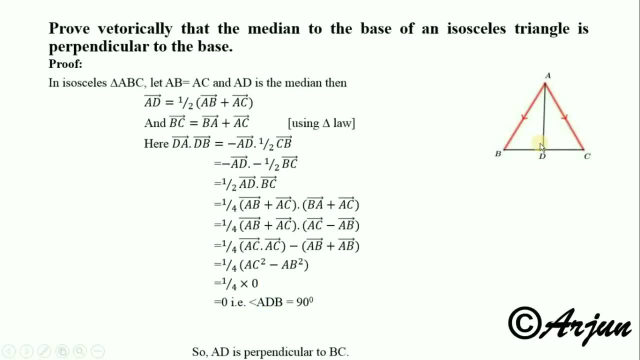 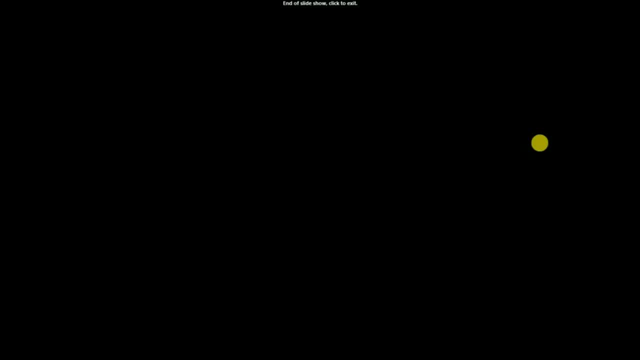 Angle AD is equal to 90 degree. Here D is 90 degree, So AD is perpendicular to BC. This is how our theorem is proved. Thank you for watching, Subtitles by the Amaraorg community. 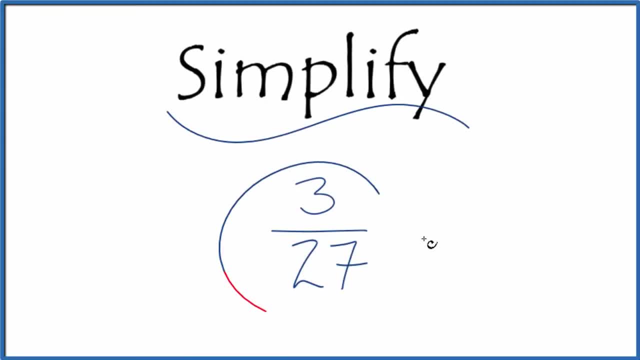 Let's simplify 3, 27s And what we're really trying to do. we want to find another fraction that's equal to 3 over 27.. It's an equivalent fraction, but we've reduced it to lowest terms. To do that, we need to find a factor that goes into 3 and 27.. I know that 3 divided by 3 is 1.. 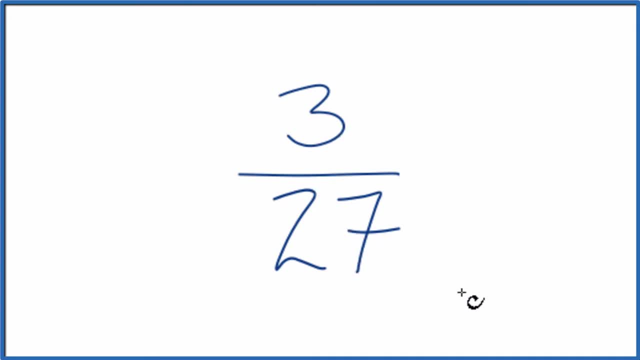 27 divided by 3 is 9,, because 9 times 3, that's 27.. So we could say 3 divided by 3 is 1, and then 27 divided by 3, that's 9.. And we've reduced this fraction 3- 27ths down to 1- 9th. 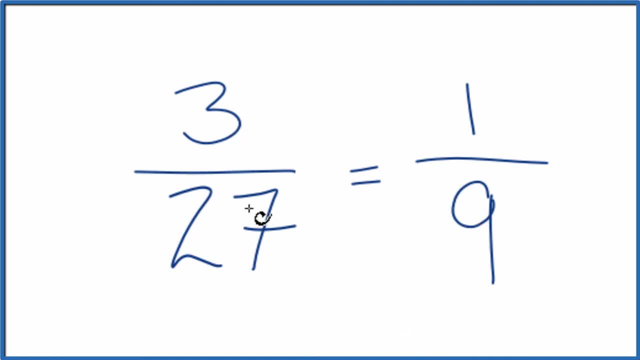 These are what we call equivalent fractions: 3 divided by 27 and 1 divided by 9, you get the same answer: They're equivalent fractions. It's just that we've reduced 3 27ths down to 1- 9th.